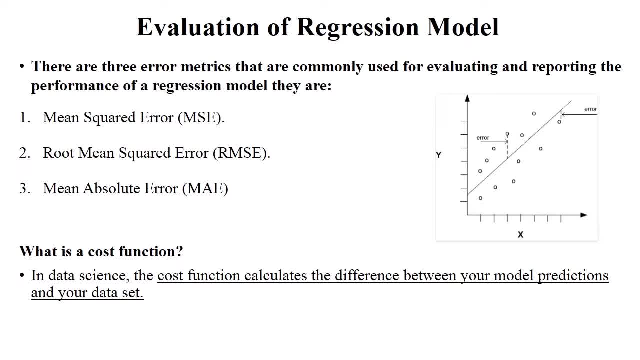 So the first point is evaluation of regression model. In our last lectures we learn the concept of regression, then concept of error and concept of list square method. So basically, regression show the relationship between dependent and interdependent variable. We took the example, that is salary and experience. right. 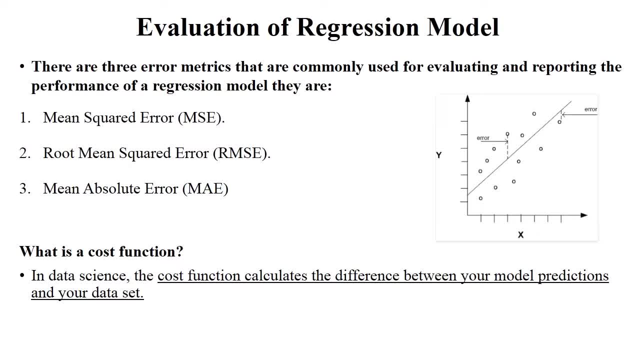 Salary is depend on experience in this way. So in this diagram, see here- Y is depend on X. It shows the relationship between Y and X. The middle line is called as actual value. that is line, and these are the. these are the predictor line. 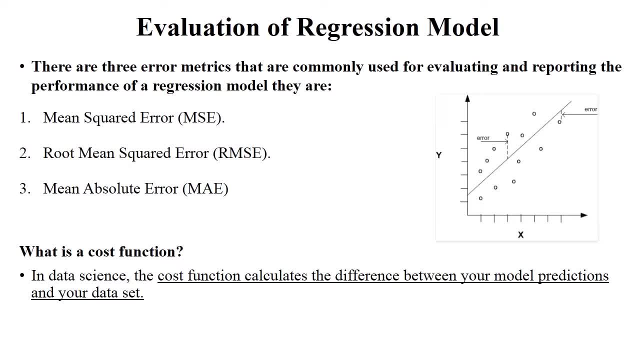 The middle line is called as predictor line and remaining are the actual values. So difference between actual value and predicted value is called as errors. Okay, so in machine learning or in regression there are three errors are present. that is mean squared error, root mean squared error and mean absolute error. 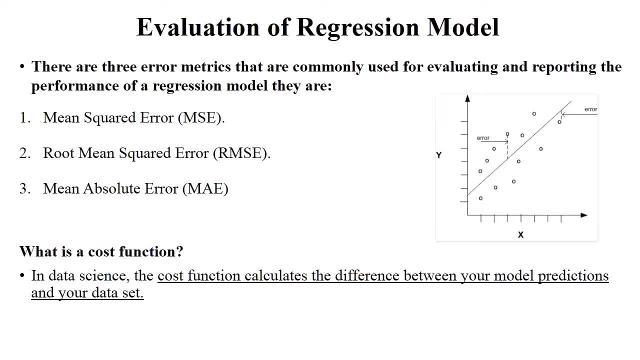 And how to how to overcome these errors. That's why we use list square method. Let's see, And this list square method We already learn in last lecture. Okay, I have mentioned the link of this video in below description box, So let's see what are the errors are present: integration. 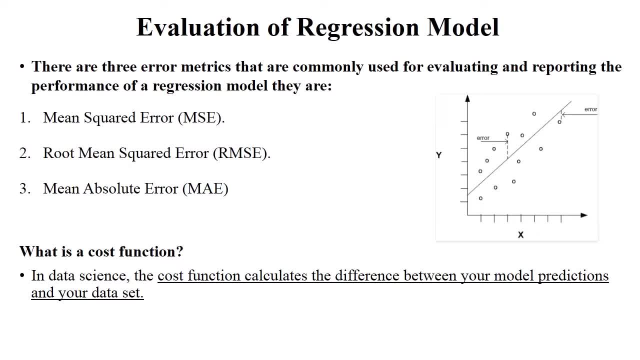 So these errors are also called as cost function. So cost function basically means to calculate the difference between your model predictions and your data set means difference between actual value and predicted value. This thing are called as cost function. and these three cost functions are there next. 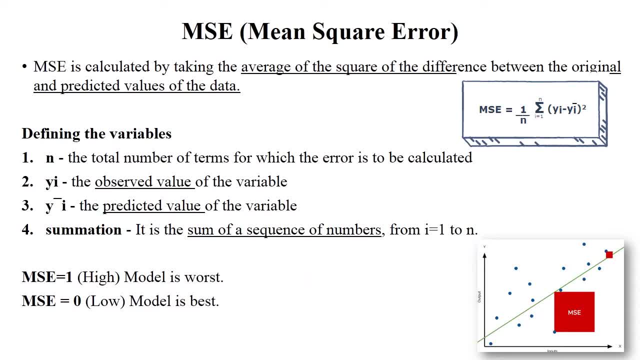 So first, First cost function is MSE, that is mean squared error. So MSE is calculated by average of square of difference between original and predicted value of data. See, in python there is directly method means mean squared error, RMSE, root mean squared error. These methods are directly used in python for implementation. 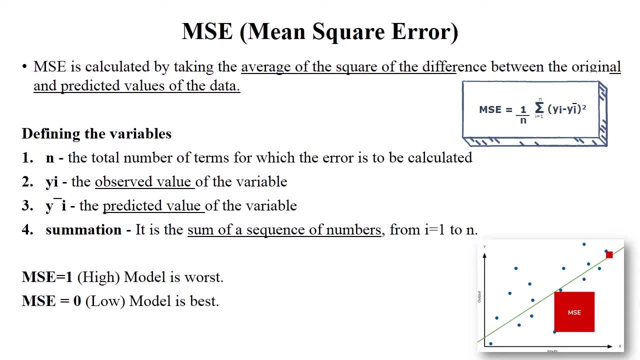 Okay, but how these methods are work, What are the formulas? are there These things we will learn in this session. Okay, so the formula of MSE, this, that is, MSE equal to MSE, MSE equal to 1 by n. summation: yi minus yi bar whole square. 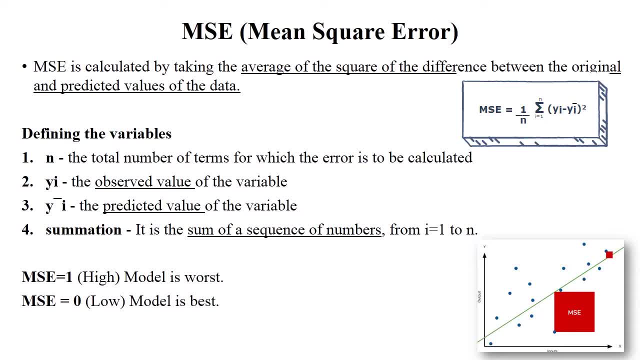 So here n means total number of values, total number of terms, yi means observed value, yi bar means predicted value. Okay, and summation means sum of sequence. So this is a formula: if the MSE equal to 1 means high, So model is worst means there are lot of errors are present. but MSE equal to 0 means MSE equal to low. 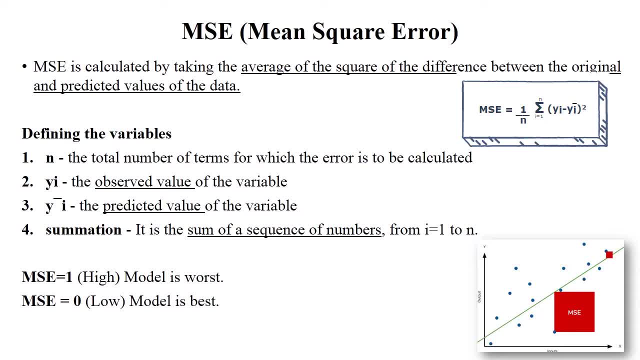 So model is best Means there is a, there is not. errors are present, accuracy is good, So this is called as MSE. see here in this diagram, This is your predictor line, green color line and blue color is actual data points. Okay, So see here there is a lots of gap, is there? there is a difference, is there? 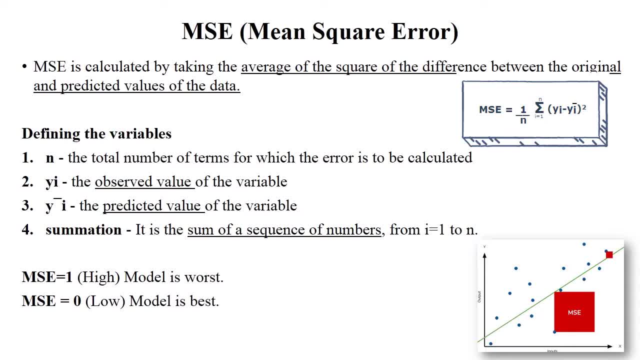 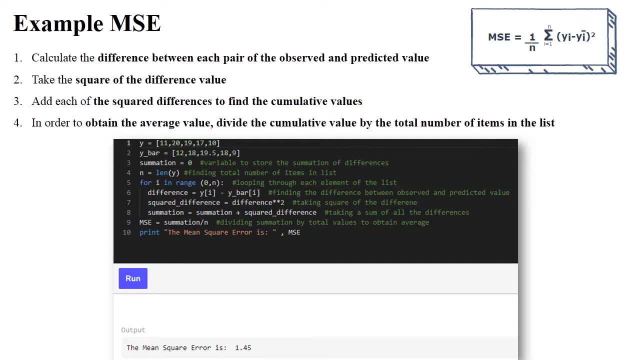 So this is called as MSE. Okay, difference between actual and predicted value. So let's take one example of MSE. So here we will implement the just formula of MSE. So this is the data of MSE in pseudocode format. Okay, see here: y equal to, there is a, one set is given- 11, 20, 19, 17 or 10 y bar- and one error is given. 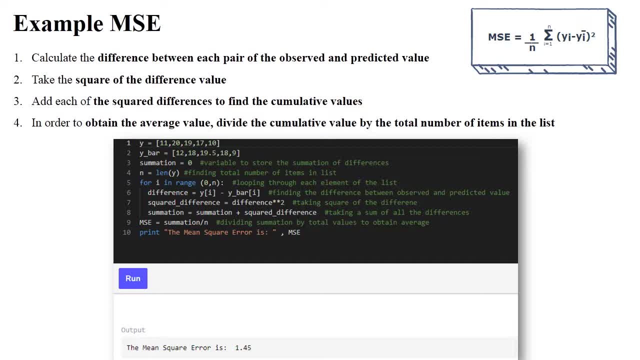 Okay, and summation at a starting equal to 0.. So you need to put up this value into this formula. For example, see here what is the formula: difference yi minus yi bar. See here: difference equal to yi minus yi bar. So what is the result of this formula that can be stored into this difference variable. 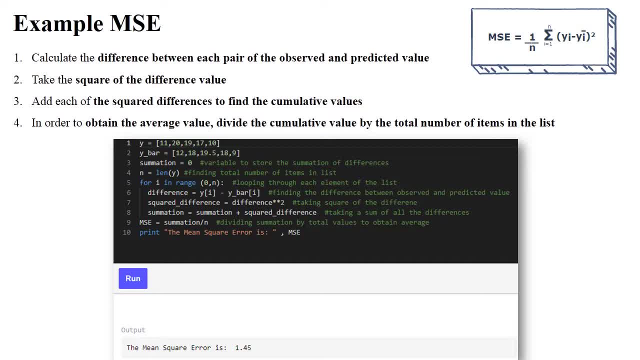 Okay. The next, this result are stored into the difference yi minus yi bar. stored into a difference and difference square: Okay, So difference square. this result stored into the variable squared difference: Okay, And after that there is a summation: plus squared difference. 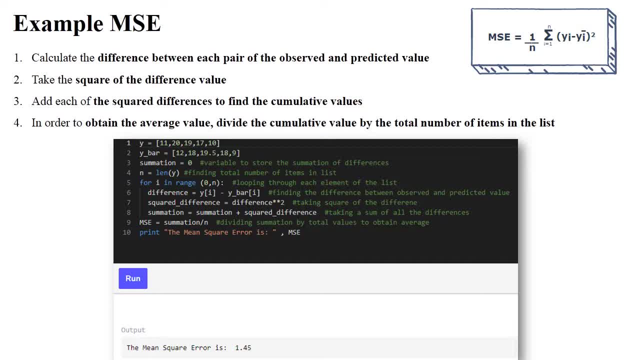 Right, So summation plus squared difference, These values are stored into the summation, So this is your MSE formula. Okay, So the difference between 11 and 12.. 11 is your actual value, but predicted value is 12.. Okay. 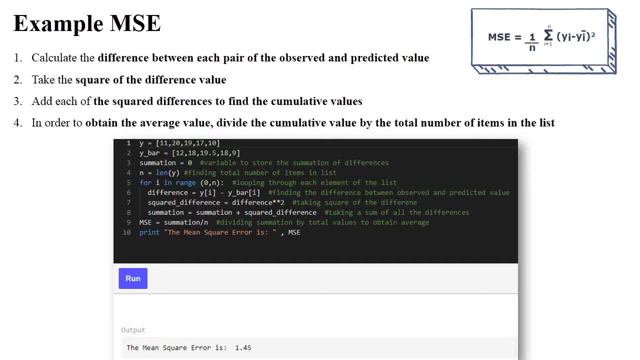 So 11 minus 12, 20 minus 18, 19 minus 19.5, 17 minus 18 and 10 minus 9 means actual value minus predicted value and summation of all those things. So this is your MSE. So after executing this program, the mean squared error is 1.45.. 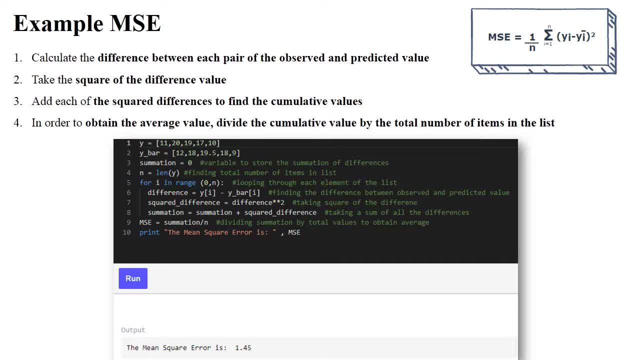 So MSE value equal to 1 means value is high. Okay, So in this way MSE value is calculated. and these are the steps. Okay, Just put up the formula and put up the all the values into the formula. So basically, there is a in Python. 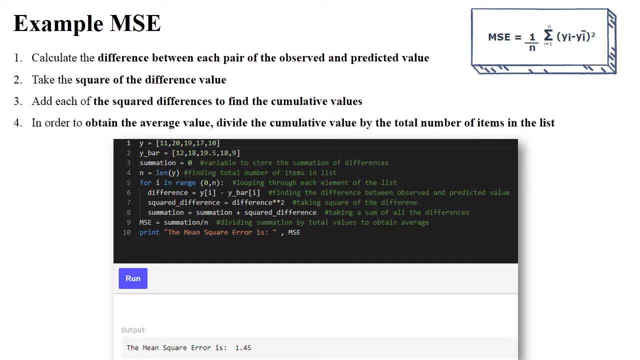 There is a mean squared error. This method is directly used, and pass the data set as a array means pass actual value and predicted value as a parameters, So this is a MSE. Now the next error is root mean squared error. This is the next cost function. 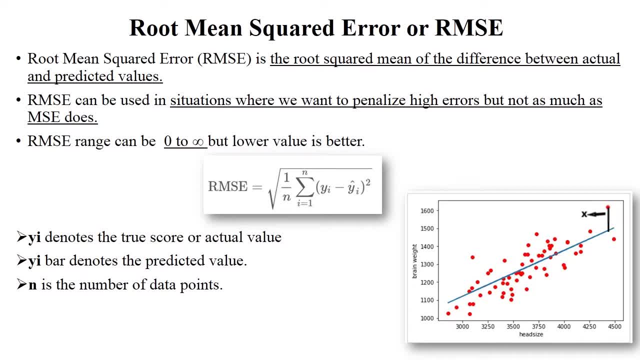 So root mean, squared error means the root, the squared mean and difference between actual and predicted value. See meaning of this. three cost functions are same, but just formula is different. Their accuracy is different, Okay, And their error rate is different, but the purpose is same. 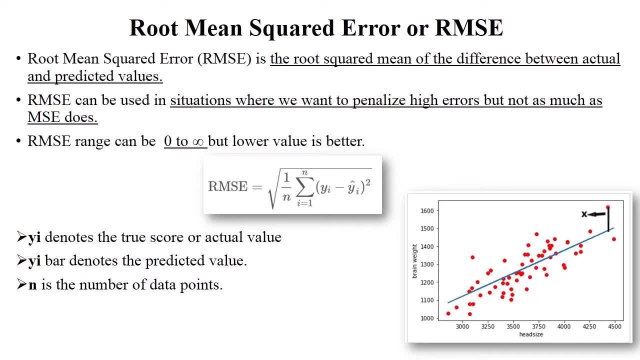 Okay, To minimize the difference between actual and predicted value. So see here, the RMSE formula is a root, that is, root mean, squared error. Okay, Means MSE formula is same, but just put up, the root is here. Okay, So same formula is there. 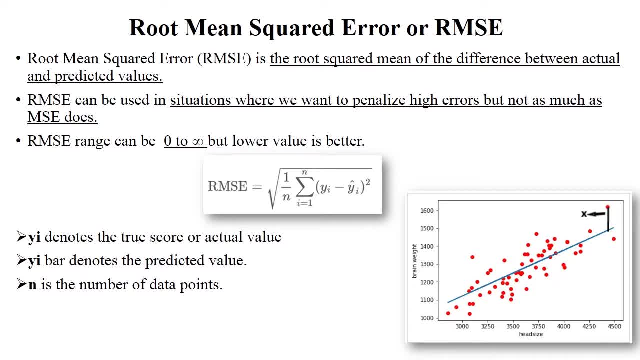 Why I minus via bar means actual value minus predicted value. So see in this diagram, the blue line is your predicted value and red dots are the actual value and there is a. some red dots are present on predicted line and there are some a difference between this. 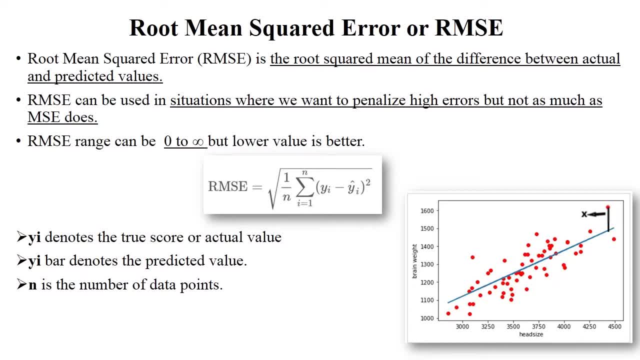 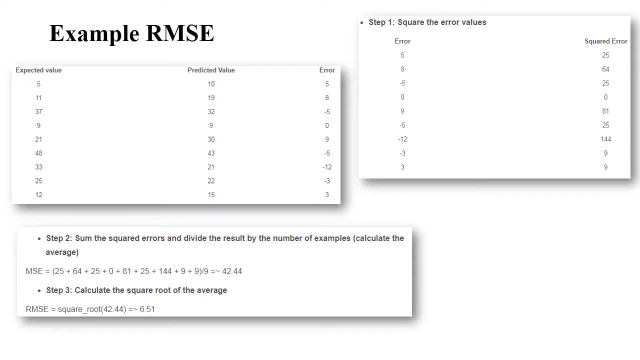 Right, So this is the RMSE, and RMSE range can be 0 to infinity, Okay, But lower value is better. So let's take one example. Okay, Now see here. Here Let's take one example in again different format. 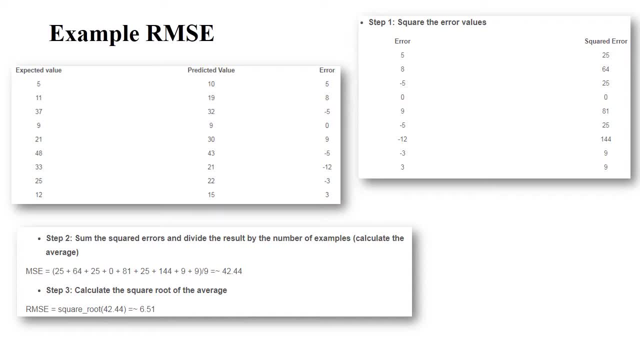 See here: Your expected value is for you, Your predicted value is 10.. Okay, So this is a set of expected value and this is a set of predicted value. So what is the error? error means difference between that. So 5 minus 10, that is 5, 11, 19. difference between 11, 19, 8 in this way. 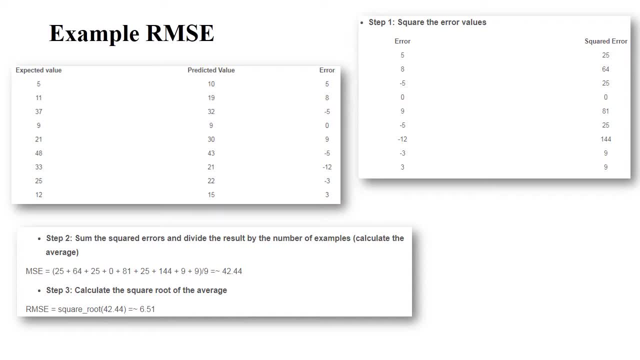 So these are, the errors are present. Okay, So see here, by using RMSE formula. first you need to calculate the squared error values. Okay, As per the formula, yi minus yi bar whole square, So answer is 5.. So square of 5 is 25, square of 8 is 64.. 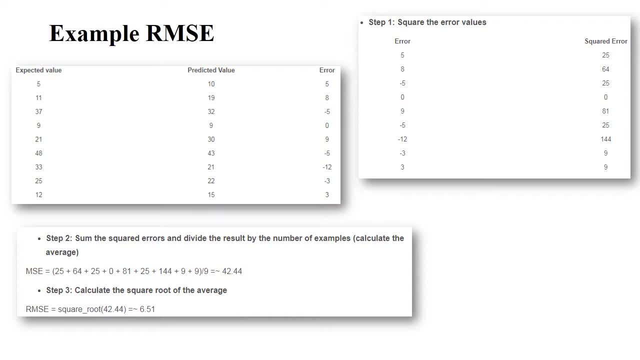 Okay, Just put up this value into the formula and calculate the squared here. Okay, The next sum of the squared error and divide the result by the number of examples. So just calculate the sum of all the squared error. that is a sum and divided by total values. 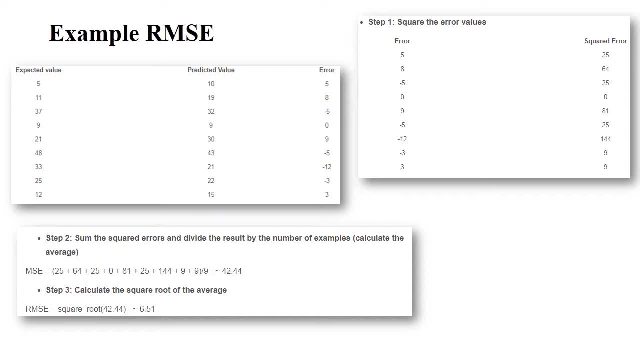 How many values are present in data set 9.. So divided by 9, equal to 42.44, and after that calculate the square root of average, because root means squared error, having the root of that particular formula Right. So square root of 42.44 is 6.51.. 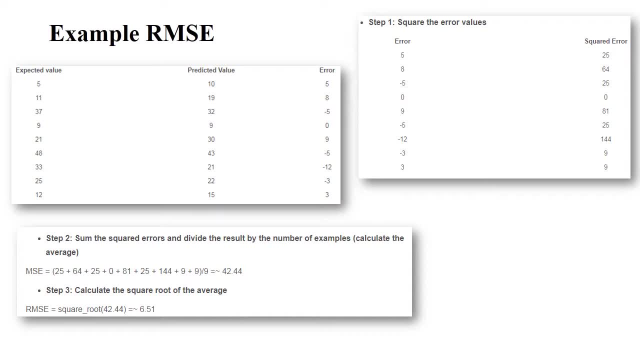 So 6.51 is average error in this particular data set. Okay, So always RMSE. answer is between 0 to infinity, but lower value is better, Right? So this is the example of RMSE. Next one is mean absolute error. 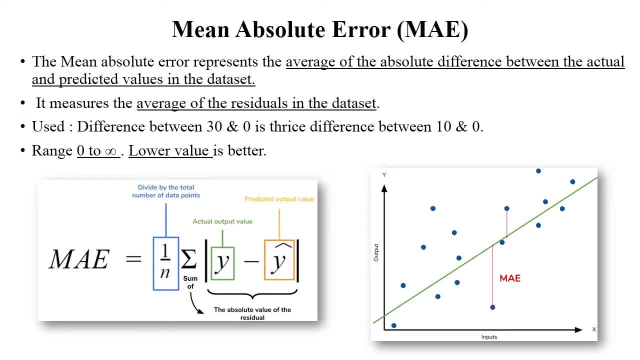 So again same, the logic is same. that is a: calculate the difference between actual value and predicted value, Okay, But mean absolute error, represent the average of absolute difference between actual and predicted value, and they use for difference between 30 and 0, a tight difference between. 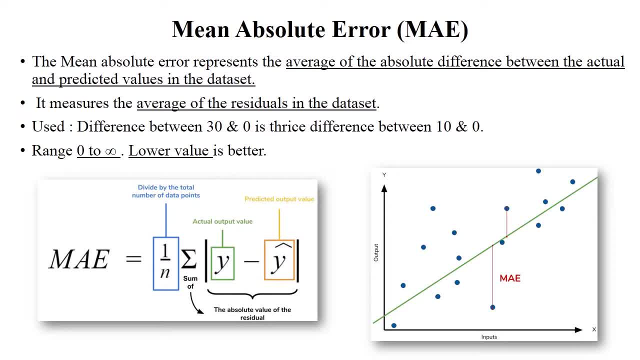 10 and 0 for this requirement. Okay, And again, their answer is: range between 0 to infinity, and lower values are greater for that. So see here again, there is a same formula, is there? Let us see What is y minus y? a bar, but there is a 1 by n. 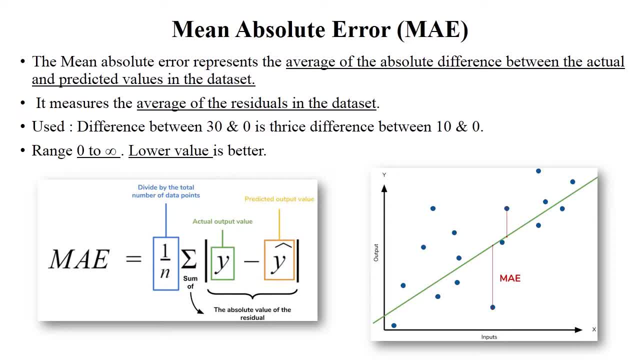 So this, these are the formula of me. This is a formula and means total numbers, y means actual value and y bar means predicted value. See, in this diagram, green line is a predicted value and blue dots are the actual value. and there is a lot of difference between actual value and predicted value. 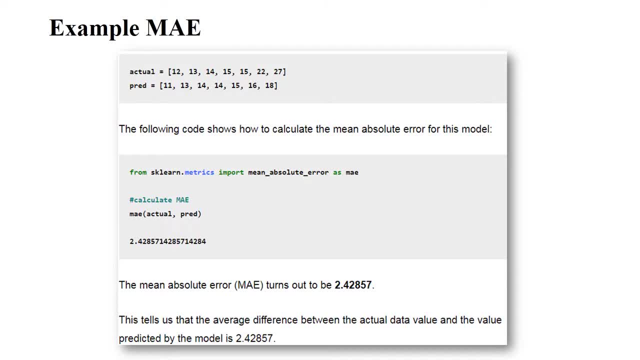 Right, So this difference is called as me Next. So see here. Let's take example in again another way. That is suppose actual value data set is given, predicted value data set is given. Okay, So while implementation of python there is, you can directly use the method that is mean. 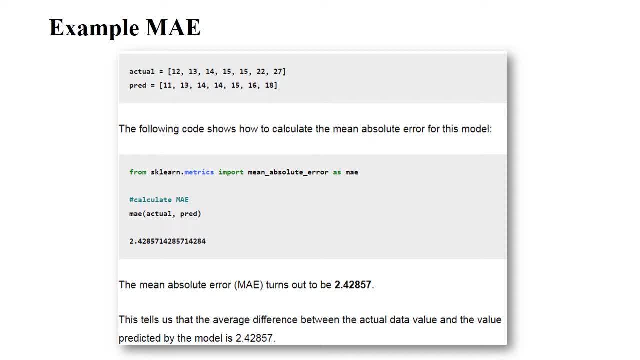 absolute error. No need to implement a formula. Okay, So mean absolute error. this method you need to import. Okay, And this method are stored into the SQL and library file. Okay, So this is a library file, This is a method.